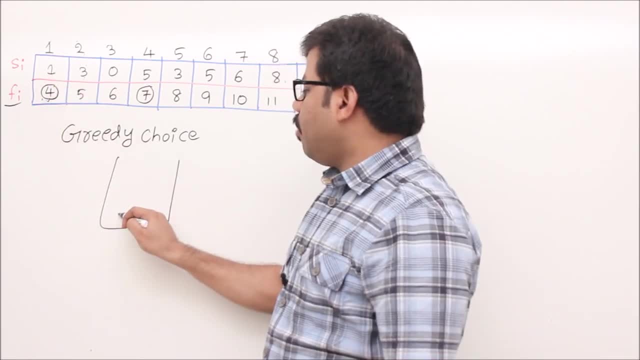 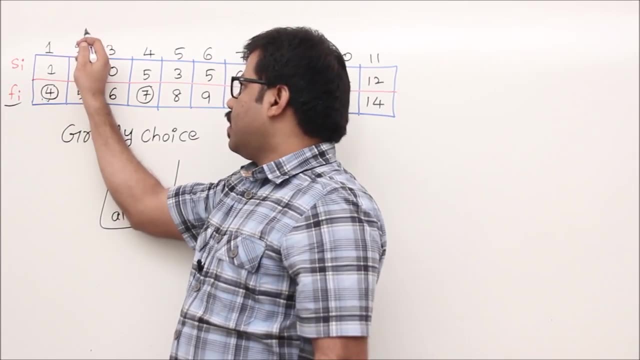 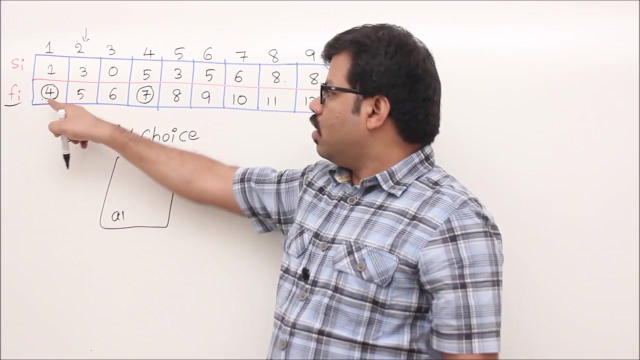 this is the activity whose finishing time is earliest right. then pick up a1. when i take it, its interval is what? one to four? then directly go right side. why you should not go left side is if you go left side, then that activities finishing times will be less than four. 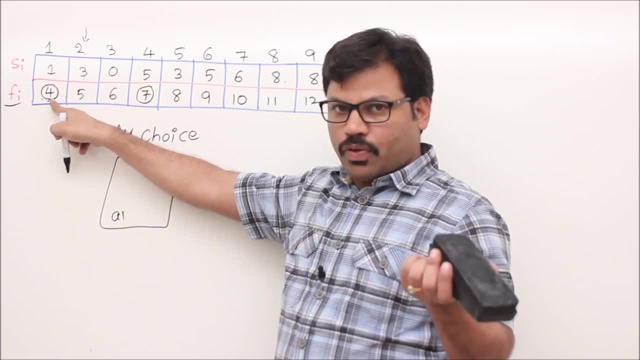 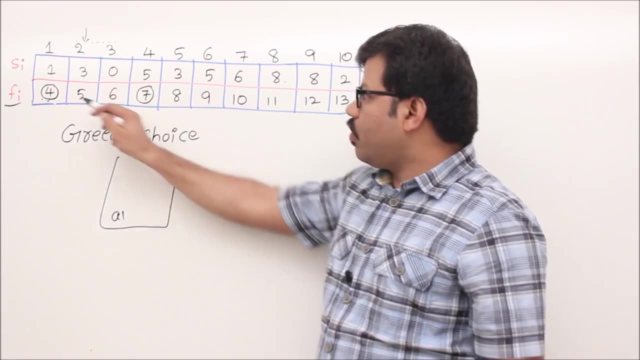 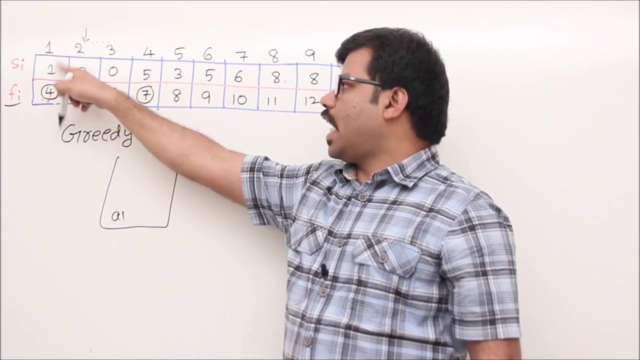 if and all if that kind of activities exist, we would have taken them before. correct, then always go right side. now start here. search for an activity who starts after four. why, if any activity starts before four, then it may not be compatible with this activity. a1 already you took a1. then your next activity. 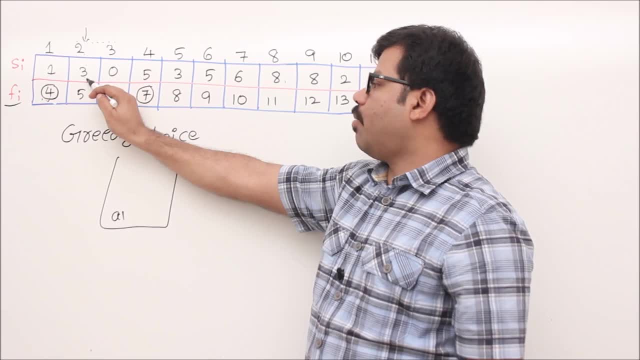 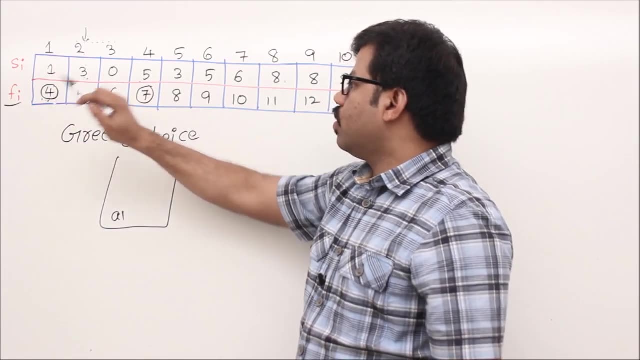 should start after four. that's why don't take this one. it will not be compatible with a1. not compatible, this is. you see, this activity starts after four. that's why take it. and especially, it is again. what is the strategy we are following? always we have to. there might be. 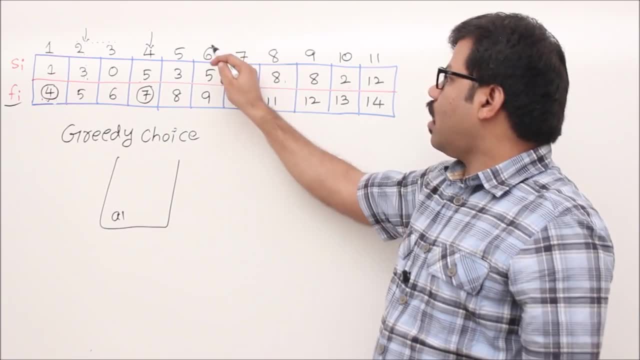 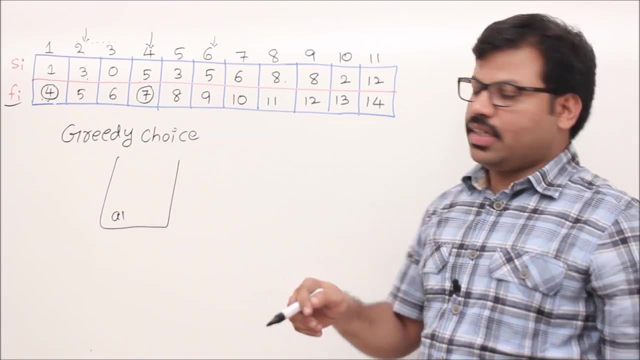 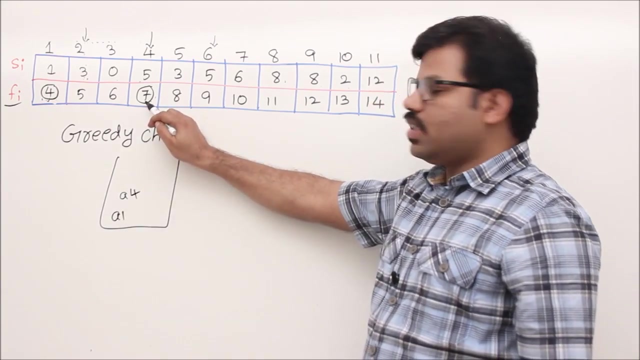 lot of such activities. at right side example. this is also starting after four, but whose finishing time is earliest. always we have to pick up an activity whose finishing time is earliest, that's why i pick up this one. then i add here a4 to the result. then this time i will fetch the finishing. 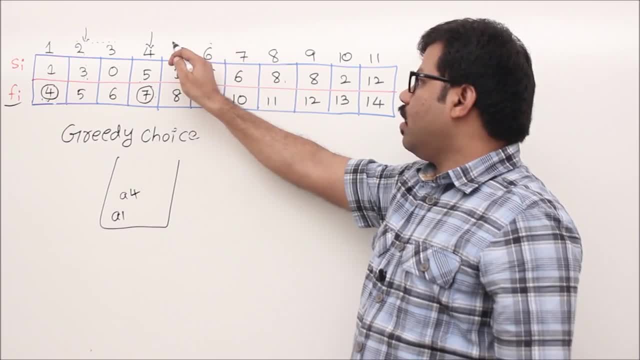 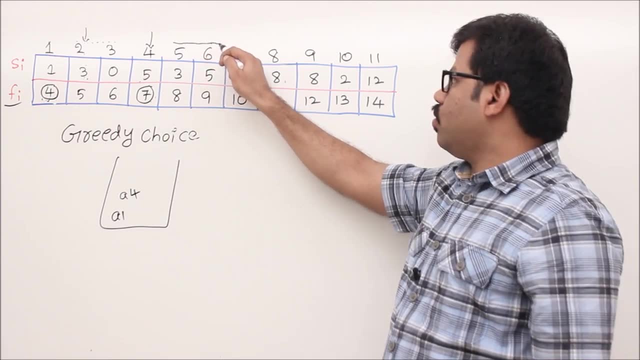 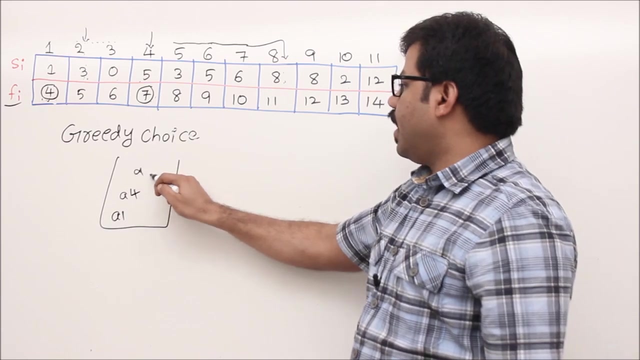 time, which is seven. this time i immediately start here and search for seven where, where i have to search whose activity starts after seven. so see the starting timings. so start time here is which is greater than seven. take it and add to the list. this is a8 and now this activity starts after seven. 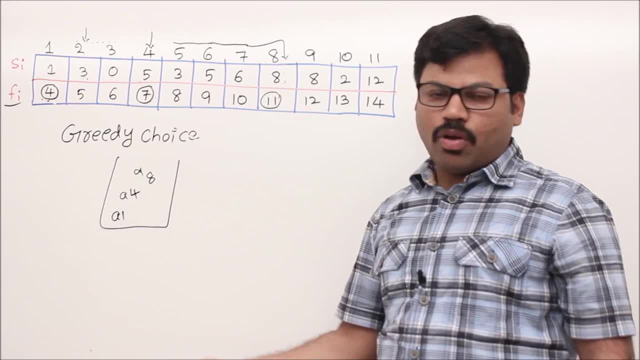 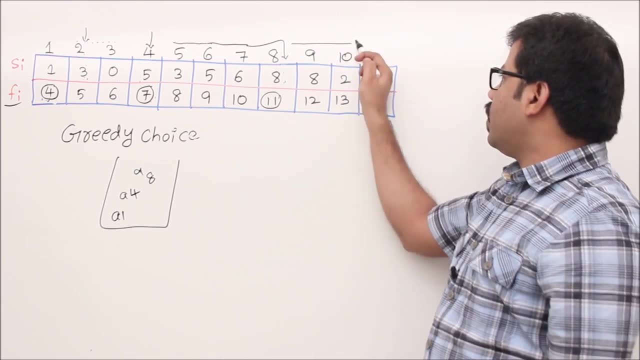 When you take A8, see the finishing time. It will be definitely earliest among all such activities. Take it This time. search for 11, immediately after 8.. Then, is there any activity which starts after 11?? Yes, 11.. 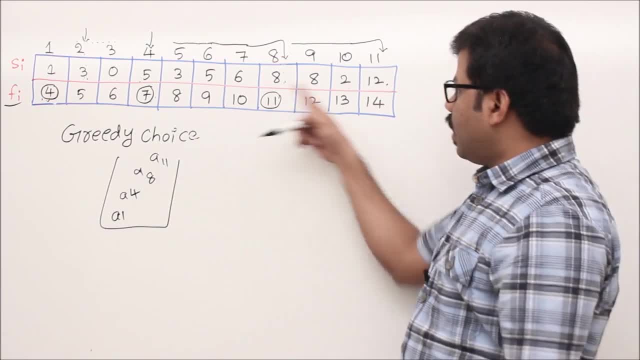 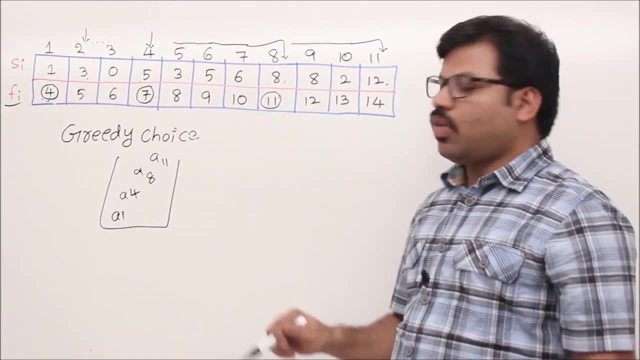 Pick it up. Do you remember one thing: While doing this strategy, we are always going forward correct, So we are not oscillating in the array. Remember that point. Now we will see the time. complexity, Definitely greedy choice will work. 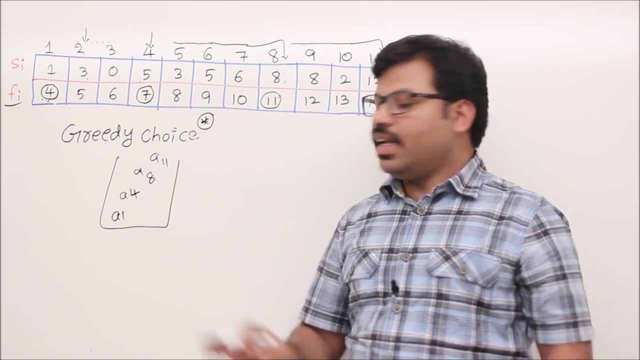 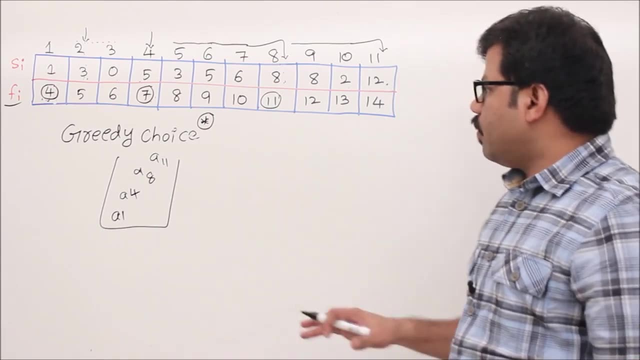 I will tell you the reason for that. Assume that, let us say, really greedy choice is working and it is giving optimum solution first, Then what is the time complexity? Now the time complexity, if you see, first of all we sorted the data. 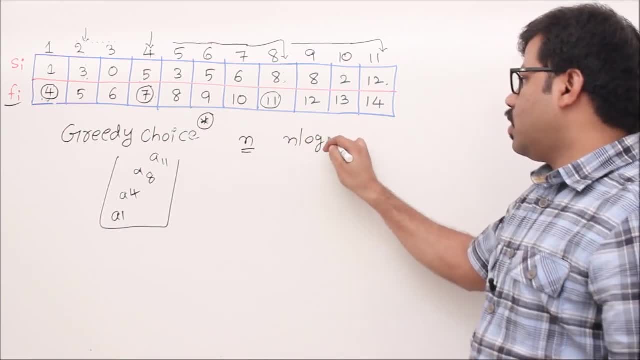 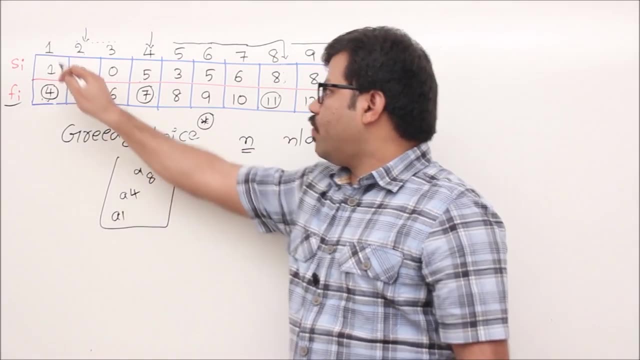 There are n activities. Then time: complexity of sorting. we know that if you use merge sort or heap sort or anything, it takes n log n time correct. Then after that take a pointer and keep it first activity. That will be the first activity which is starting. 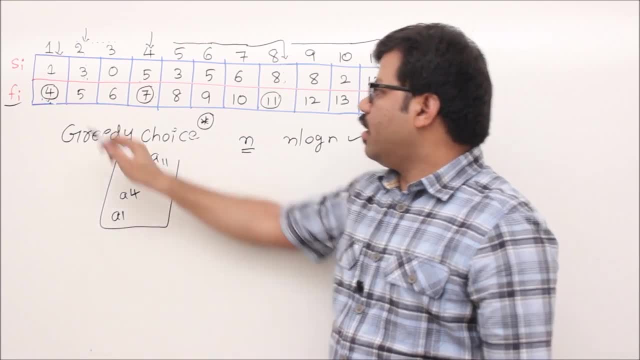 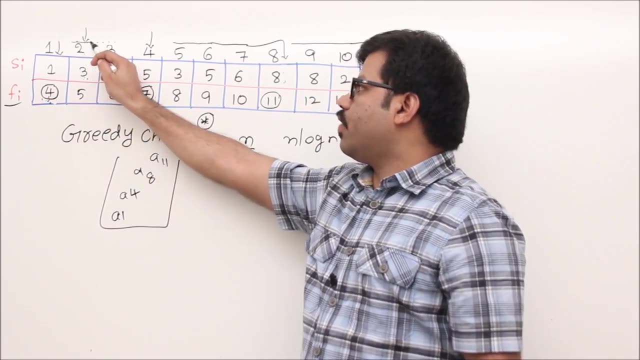 I mean whose finishing time is earliest. Take it, Then finish So it is the finishing time, And search for an activity whose starting time is after 4.. But go right to left. in that way, While searching, you will come away somewhere and take that activity and fill here. 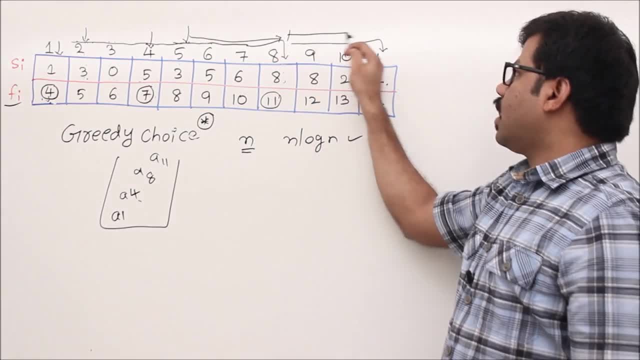 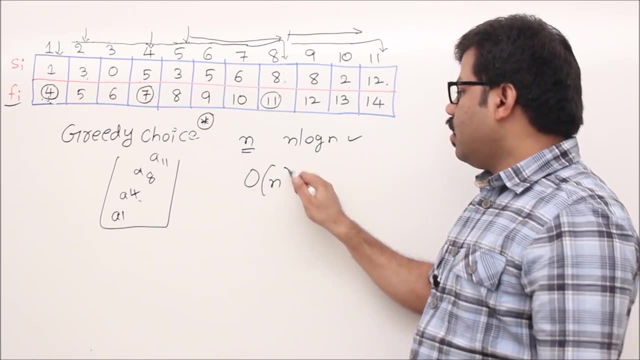 Then again search here for the next activity. Again search the next activity here. Eventually, what I am saying is: so your total program's running time is only order of n, The reason we are simply scanning your array only one time, right. 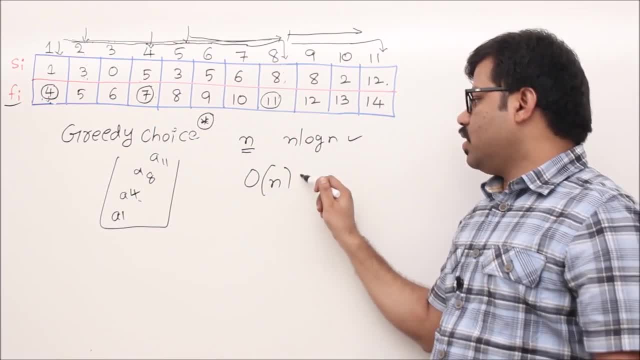 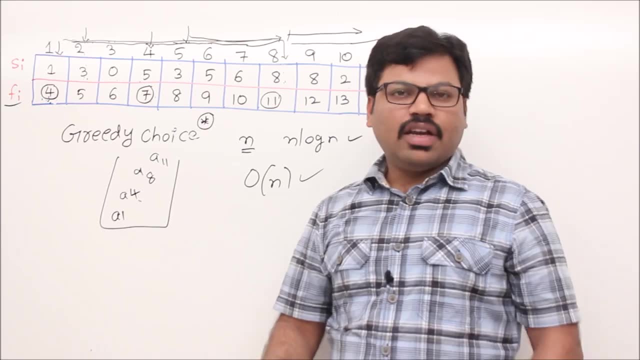 So always we are going like this. That is why the time, complexity, That is the order of n correct. So when it will be more than n example, always for every activity I took, let us say one activity. 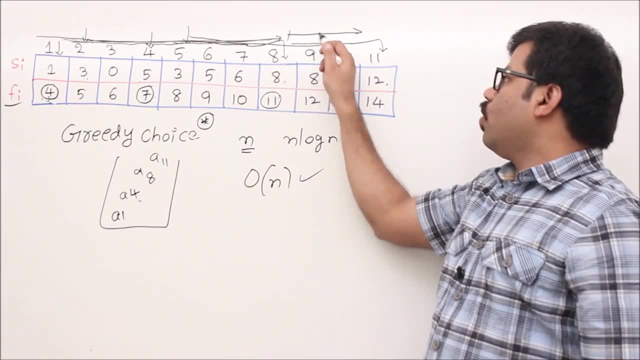 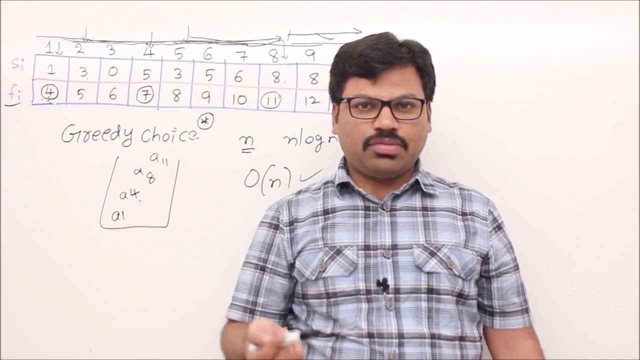 After that, again, if I start from the scratch and again, if I go up to n, then the time complexity will be order of n square, Because you will be, in the worst case, doing that activity n times. But here what I am doing is when I select an activity so I travel for some point, correct? 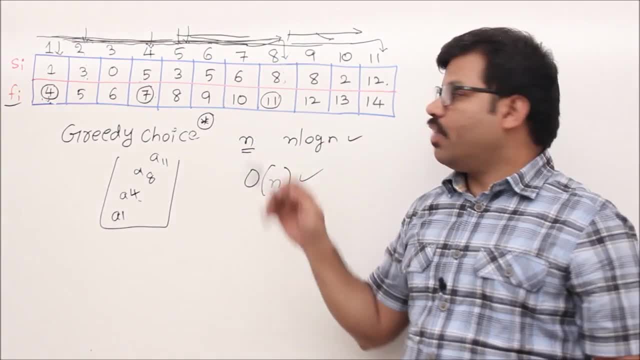 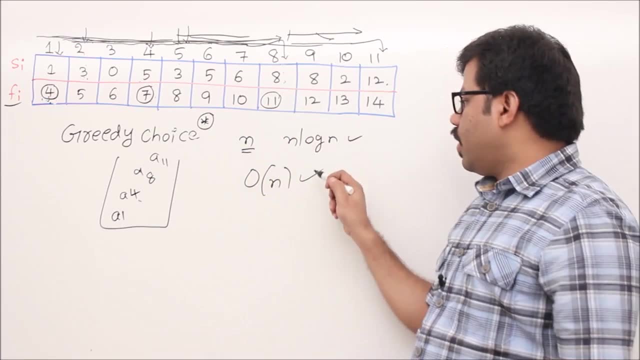 After that my search begins at right side, correct? I never come left again. That is why, If this, at most you are traversing entire array, not more than that. that is why algorithm time complexity order of n, but for sorting the data, n log n: okay. 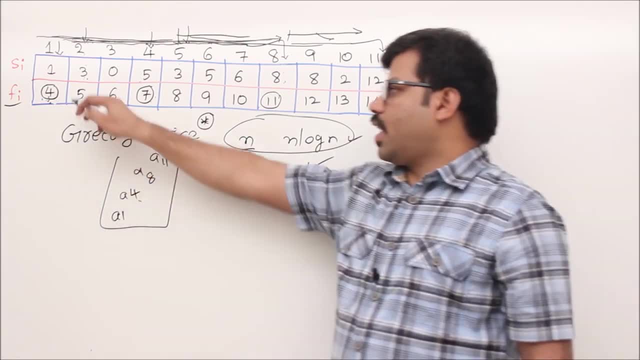 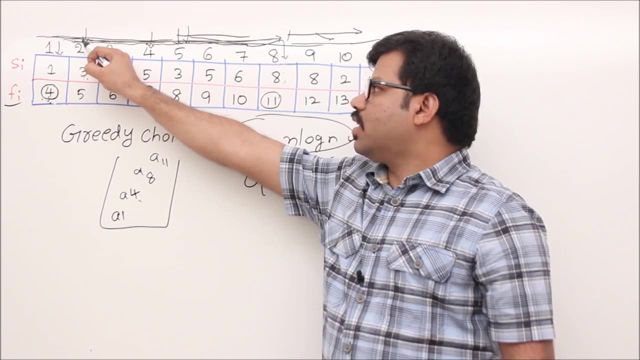 Now let me revise the solution. Take the first activity, a1, and see the fetch, the finishing time 4.. This time start at second activity. search for a value 4 in the start times. We stop here, see. 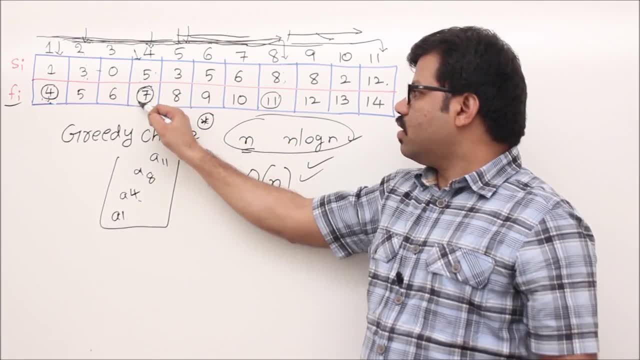 So we are just searching the array, that is it. Now immediately fetch the second dimension, which is 4.. Now we have to find the third dimension, which is finishing time, which is 7.. Now start at the next location and again search for 7 or greater than 7.. 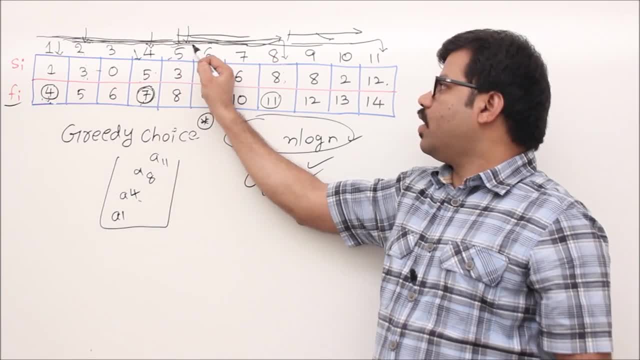 We stop here in that way. So we are after all scanning the array, that is it? Not more than that. That is why. order of n, Did you remember? So dynamic programming solution first, order of n, cube Now we got, since we have greedy choice. that is why. 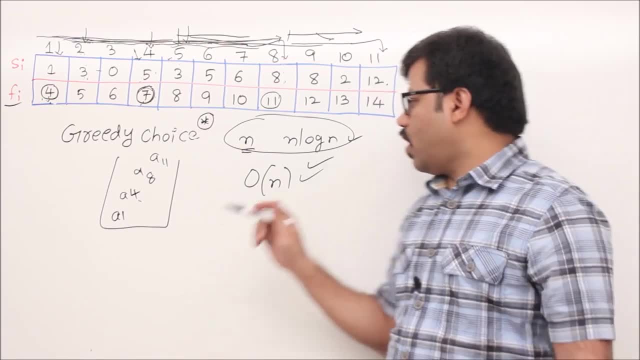 Greedy choice won't work for every problem. Don't say that, sir. I solve every problem using greedy technique. It won't work. Greedy technique can be applicable only if that problem is solved. So we have to solve it. 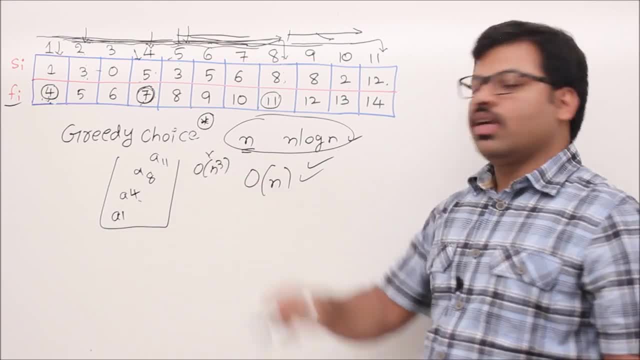 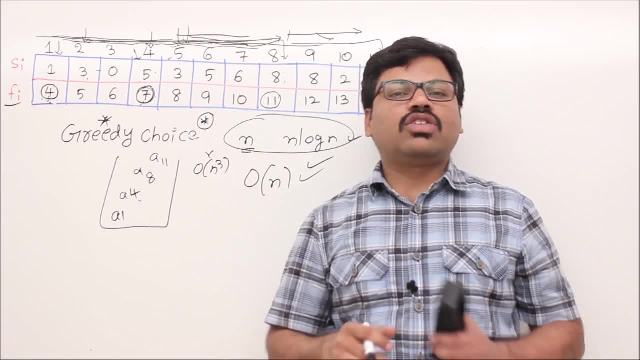 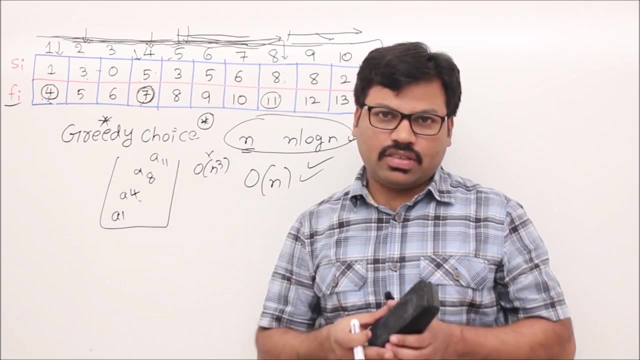 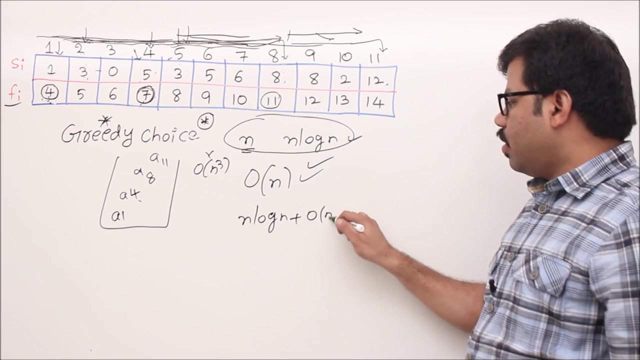 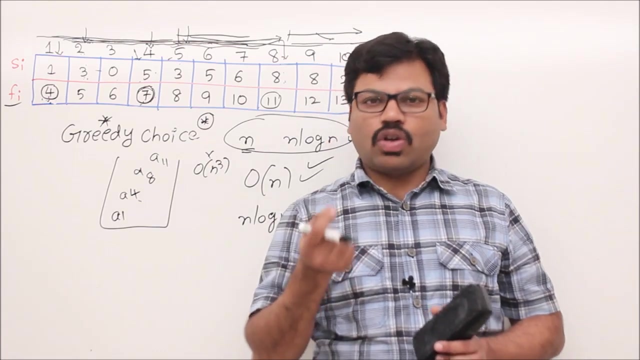 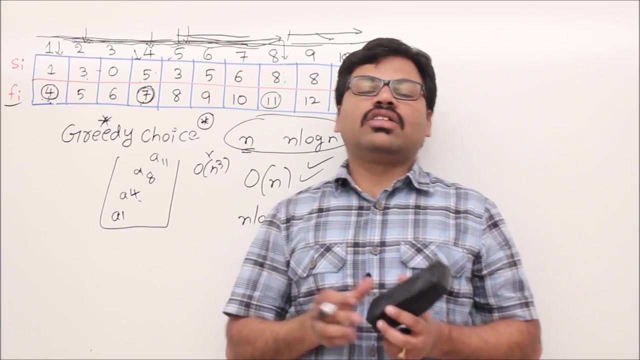 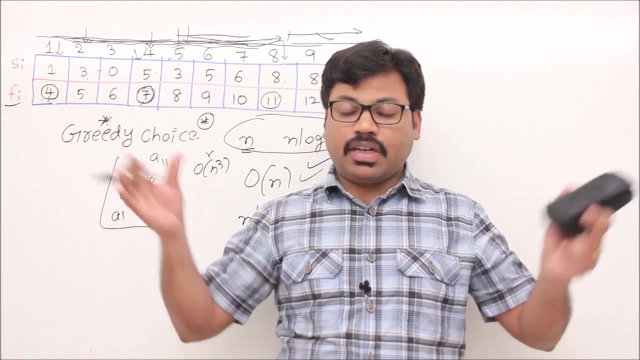 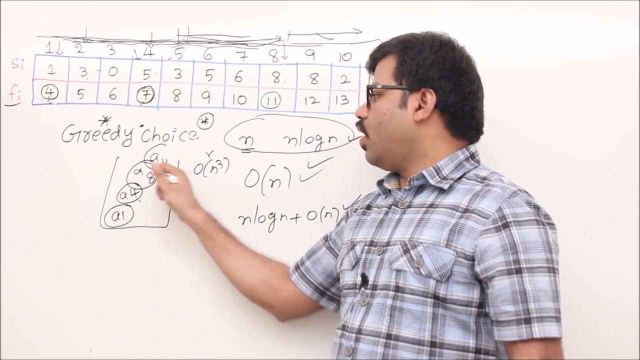 So we have to solve it, าน arbe, and you solve it, then you can solve it better than dynamic programming. understand so. and the difference comes because dynamic programming was considering all possibilities, but greedy technique was only considering best choice. that means only one choice: it was fixing and 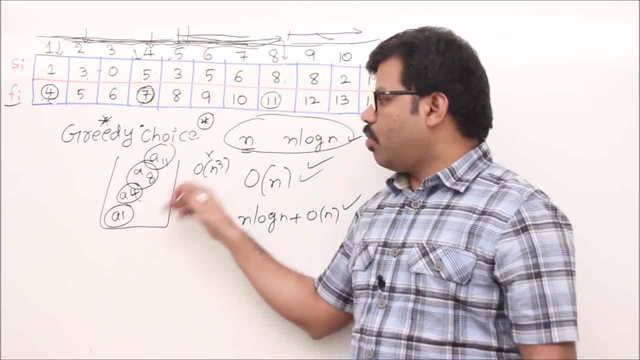 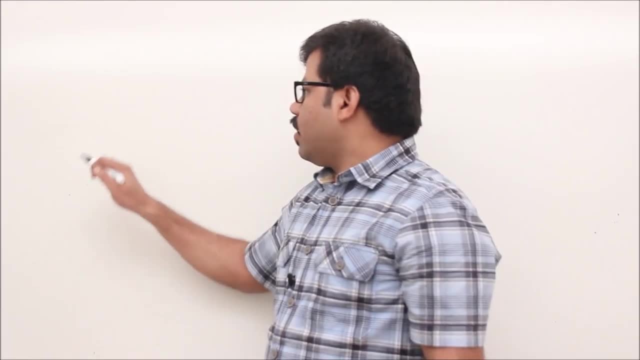 it is hoping that it reaches to optimal solution. but in this problem it is reaching, but not always understand. now we will see why this greedy choice always gives optimal solution. so for that i take, you know, two solutions. one is my solution, second one, let us say, optimal. 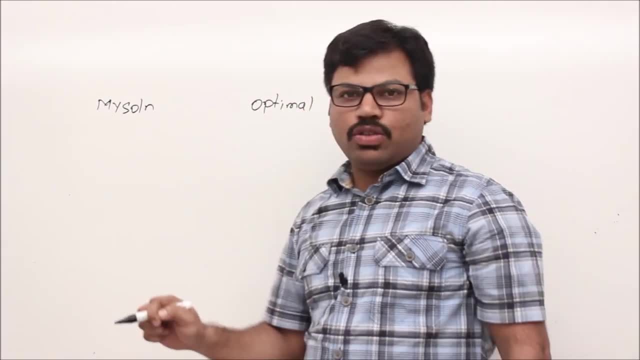 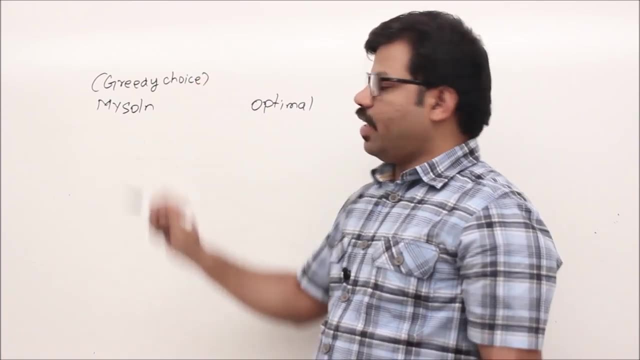 solution and i am assuming that initially my solution, which is using greedy strategy, that means which is using greedy choice technique, is not optimal. let us say first, i assume it is not optimal. after that i prove that it is optimal. so this is, let us say, optimal solution. 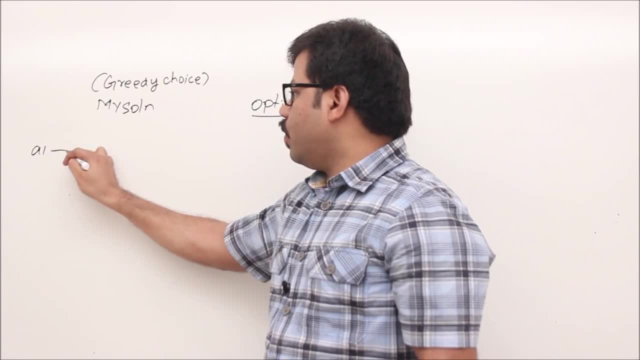 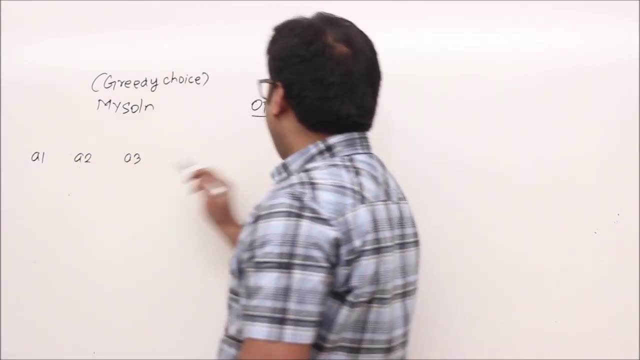 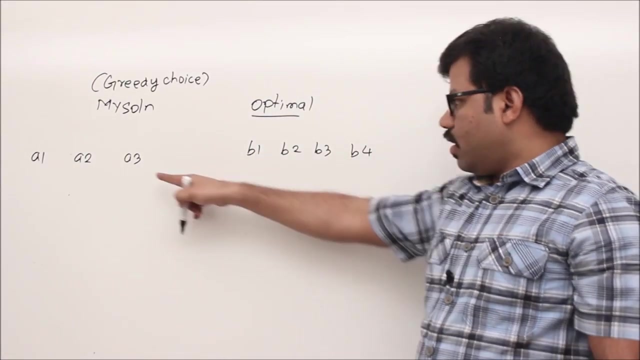 my solution is not optimal, but i know the activities in my solution, that is, one is a, one, optimal after that a2, after that let us say a3, and optimal solution has activities b1, b2, b3, b4. so definitely at least one more activity optimal solution should have. right then, only it is. 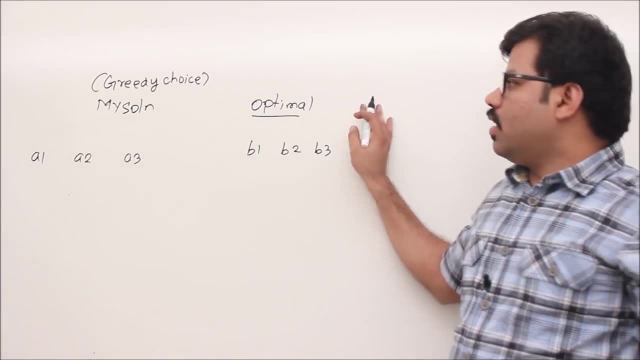 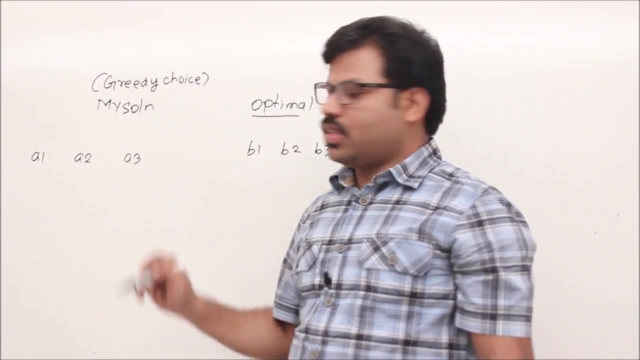 optimal. if this also has three, then we are same. then i can say that my solution also optimal, correct with respect to number. now let us say it has four activities. i have three activities. first of all, i compare a1 versus b1. if they are same, then i compare a2 and. 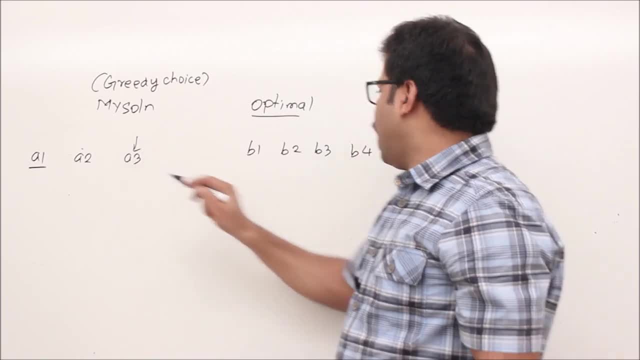 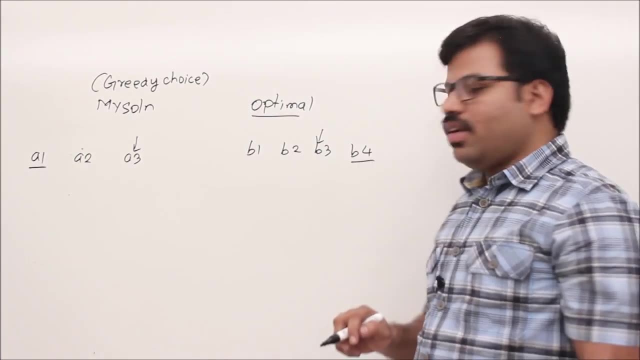 b2. if they are same, then i compare a3 and b3. if they are same, if a1, a2, a3 equal to b1, b2, b3, then he picked b4, right? if he can be picked before, then i also can pick one more. 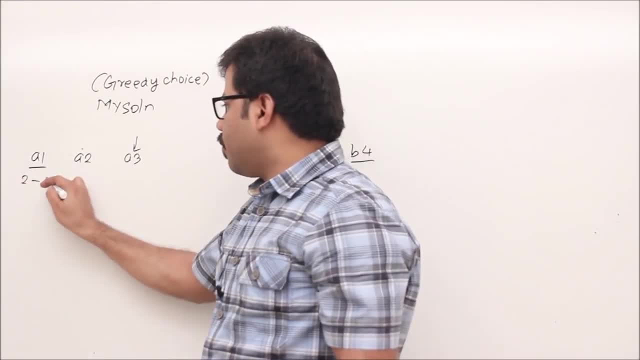 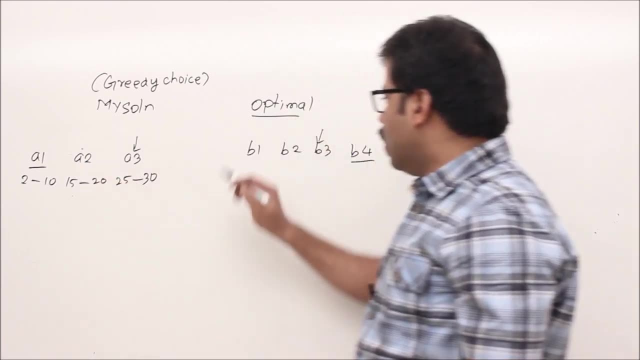 candidate, isn't it why? example: a1's activity, 2 to 10, a2's activity, let us say 15 to 20, a3's activity, something 25 to 30, see all are compatible, since b1, b2, b3, equal to a1, a2, a3. 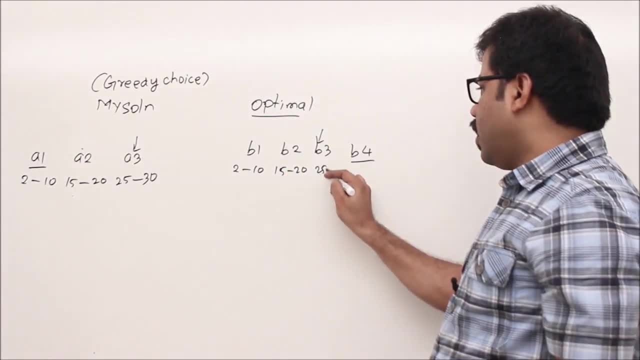 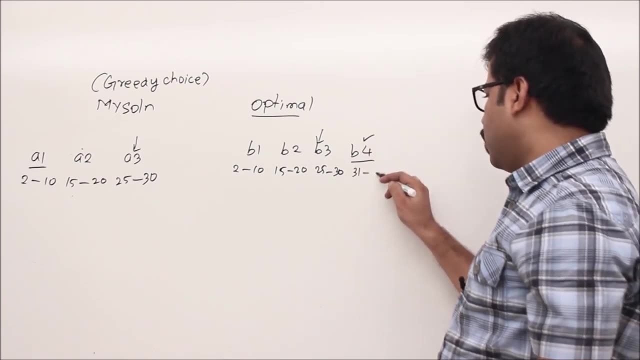 they will be 2 to 10, 15 to 20.. so all are compatible: 20,, 25 to 30.. Now, if B4 he can pick, then that's starting time should be after 30, maybe 31 to something, 50 or something. If he can pick it, then according to my greedy choice, 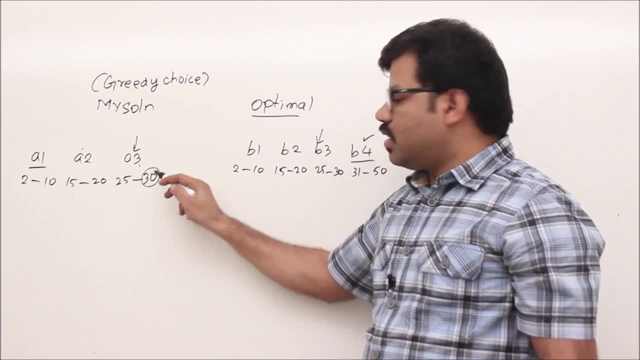 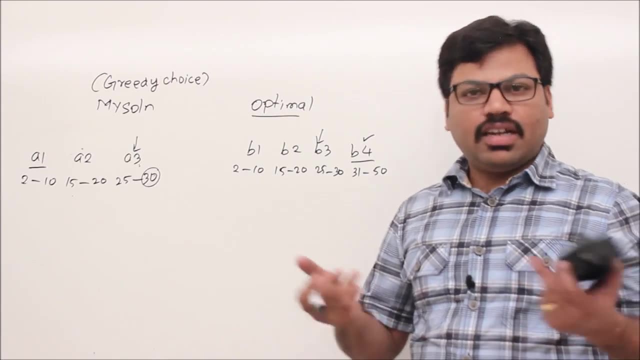 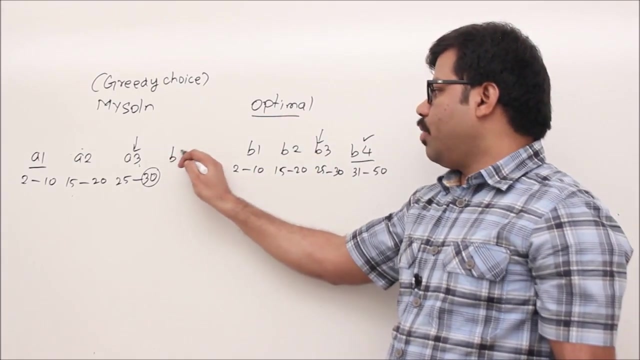 after picking A3, whose finishing time is 30, I search for activities after 30. If he can get an activity, I also can get activity, because both are working on same set. That's why he is wrong. That means really he is getting B4, I also get B4, then my solution also optimal done. 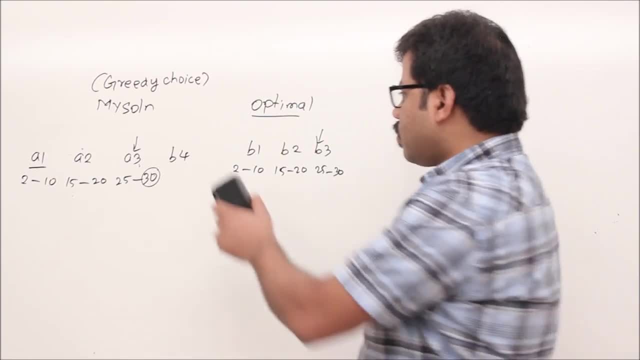 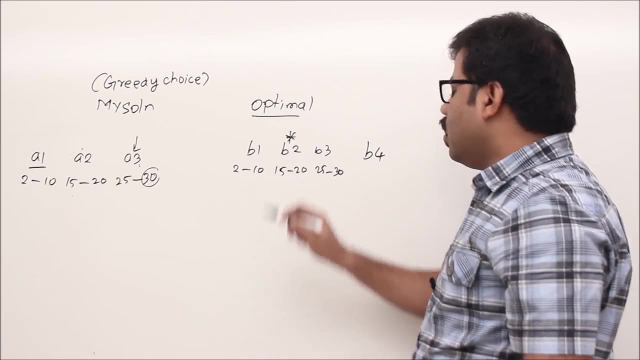 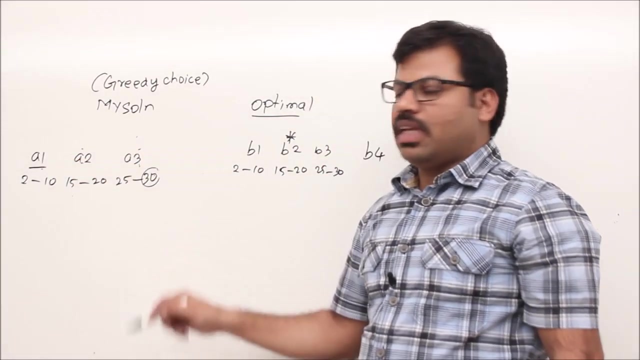 So second thing: maybe he has four activities, but before B4, let us say, here there is a difference. I took A1, A2, A3,, he took B1, B2,, B3, B4, but not all are same. That means his activity is A1,. 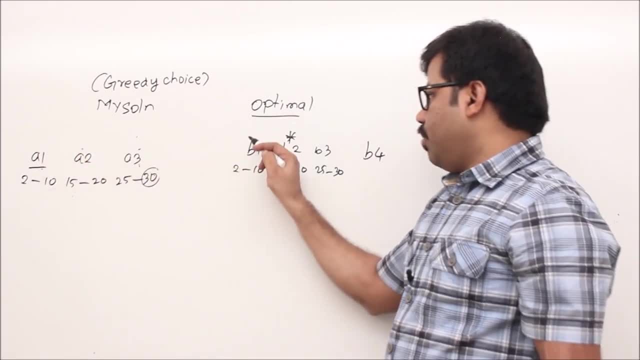 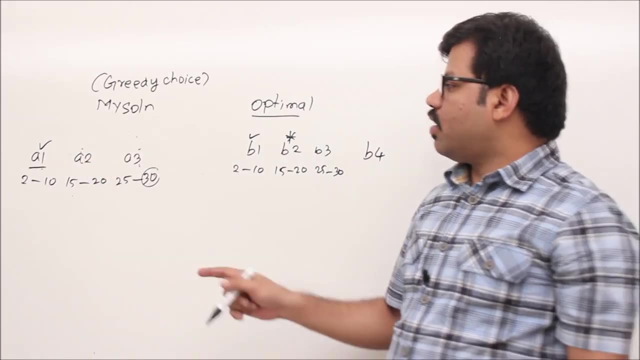 I mean, my activity is A1, his activity B1, it matches, but A2 does not match. That is second possibility. First one: what we did, we thought A1, A2, A3 matches with B1, B2, B3, but in that case we proved that that 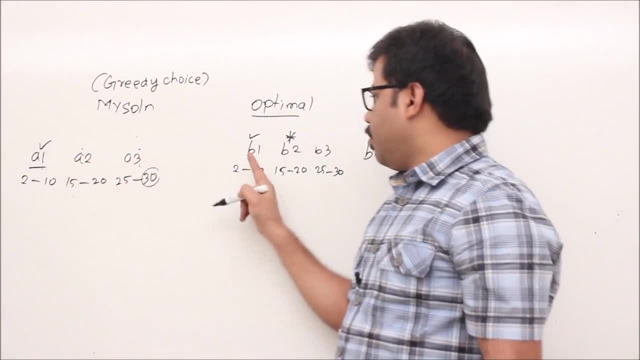 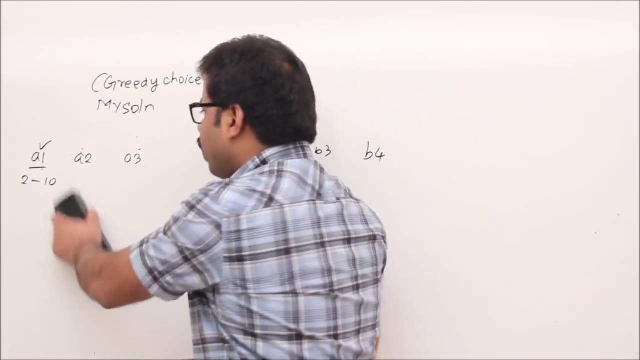 is impossible. Second one: if A1 matches with B1, but A2 and B2, let us say first time they differ- then I ask: we will see If they differ. what are the time intervals? A1's time interval. 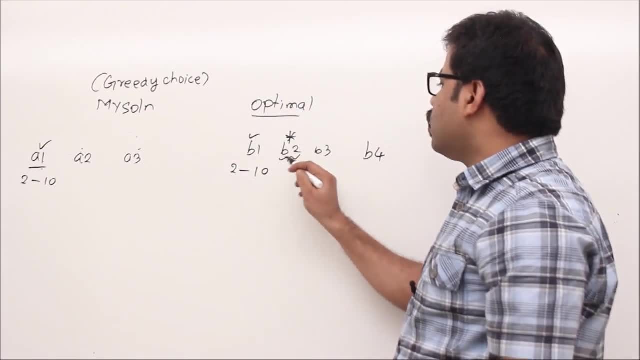 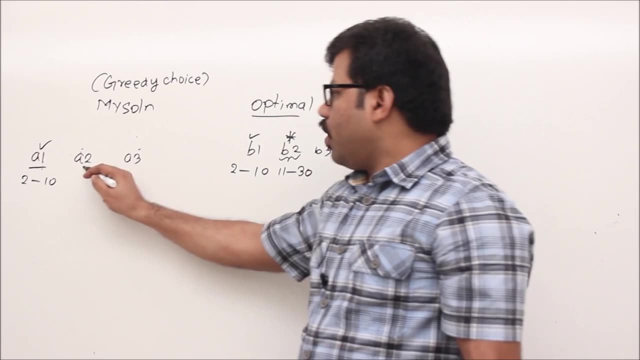 if it is 2 to 10, B1 also 2 to 10.. Then what should be B2's time interval? B2's time interval should be after 10, correct? Maybe 11 to 30 something. Then what about A2's interval? 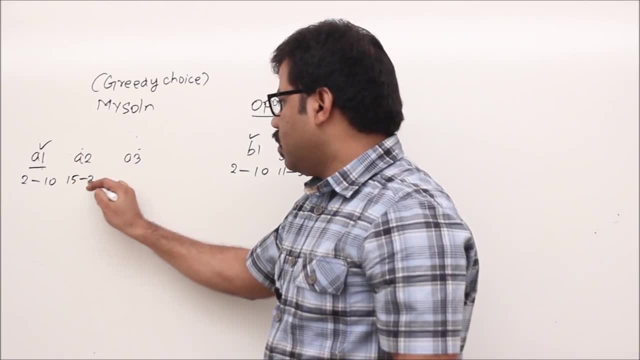 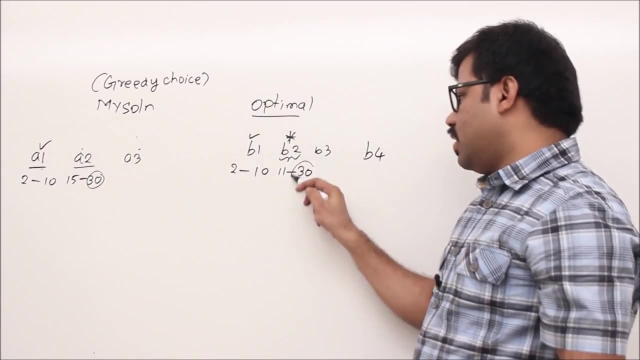 If it is, let us say 15 to something 30. Then both are. see A2's time interval finishing time is 30, B2's finishing time is 30. Now did you remember? in greedy choice, always we pick up. 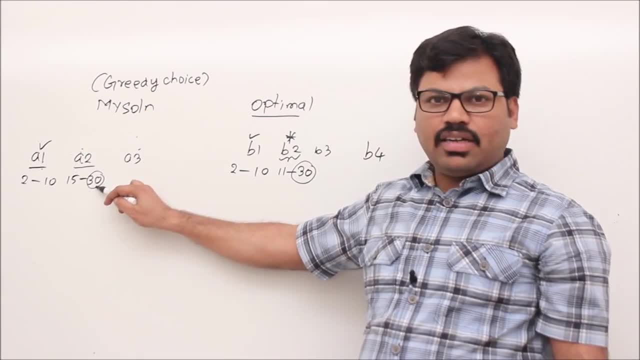 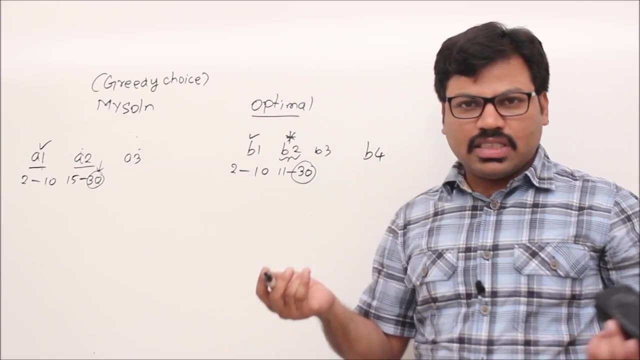 an element whose finishing time is earliest. correct. So here, according to my greedy choice, if I in the place of A2, I would have taken this one also. I had a possibility, correct? That means so really I did not pick. B2 means what? 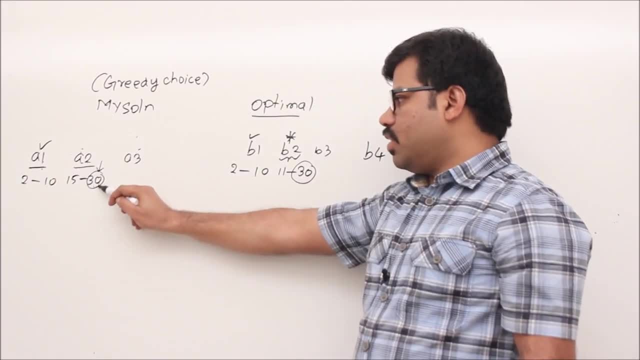 There are two choices for me at that time. One is: A2's finishing time is 30, B2's finishing time 30, that is why I picked one thing Instead of this one. I would have picked B2, correct? Not? 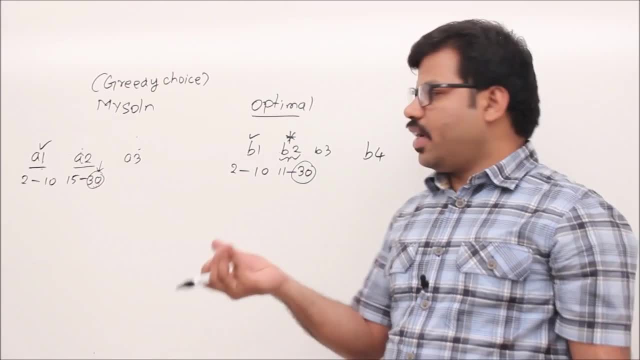 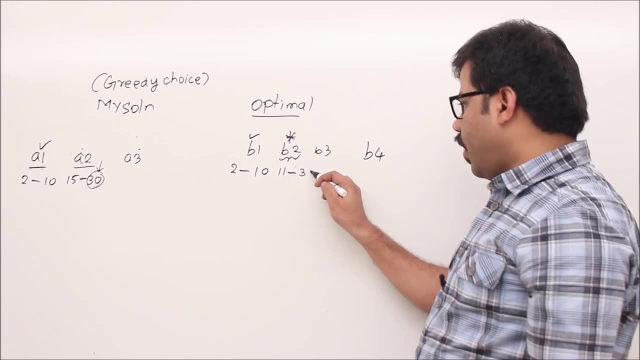 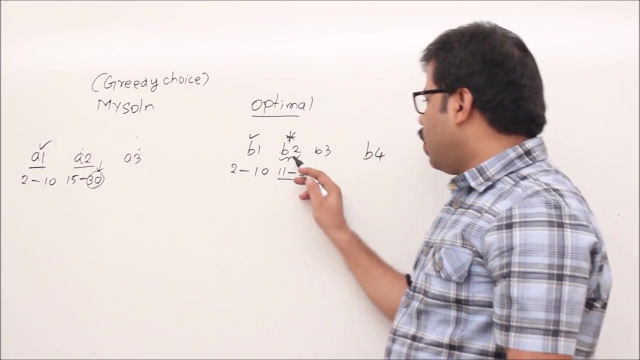 a problem for me, That means I was capable of doing that. okay, Let us say not a problem. that is not a problem. still, I am right. What if it is 11 to 35?? Then, if this is the case, your finishing time is 30, B2's finishing time is now we. 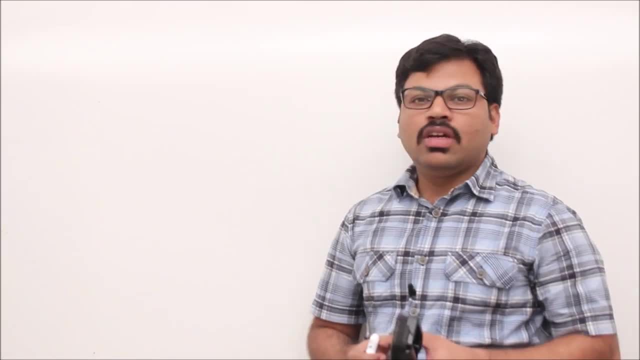 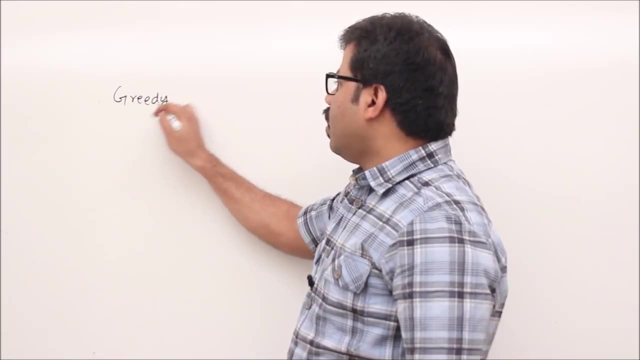 will see why greedy choice definitely now. we will see why greedy choice definitely leads to optimal solution. Let us take two methods. one is greedy method, second one another method. I do not know what is that method. Greedy method is my method and another method. 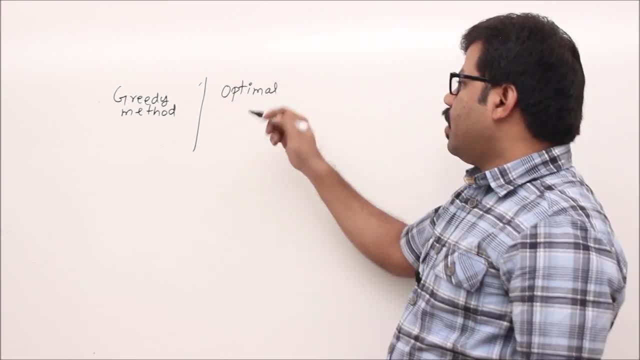 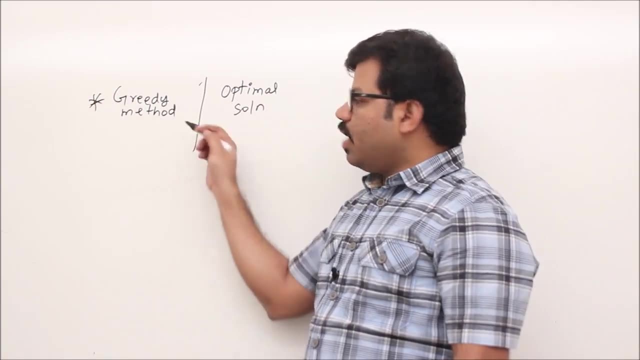 is, let us say, optimal method, That means it is giving optimal solution. Assume that, let us say, your greedy method is not giving optimal solution, but I prove that greedy method always gives optimal solution. Okay, first of all, list out all the activities. 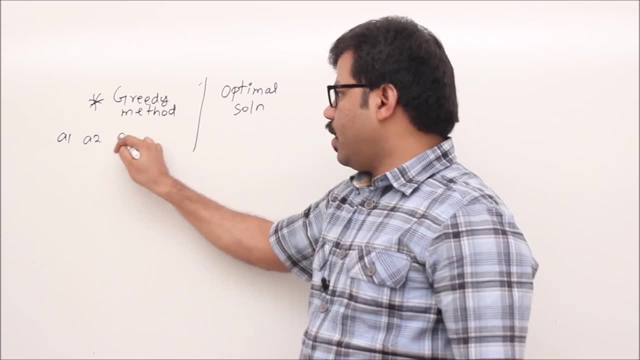 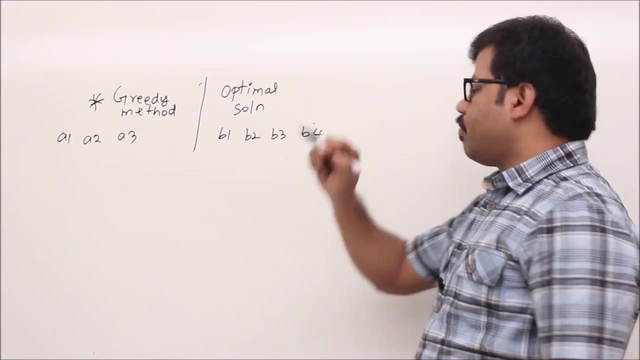 in your greedy method They are, let us say, A1, something A2, A3. So here optimal solution should contain at least one extra activity, that is, let us say, B1, B2,, B3,, B4. Otherwise, 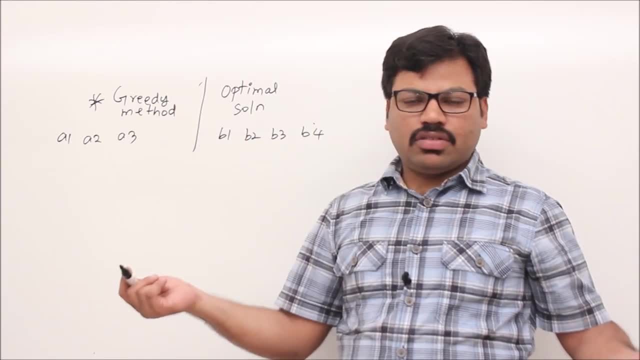 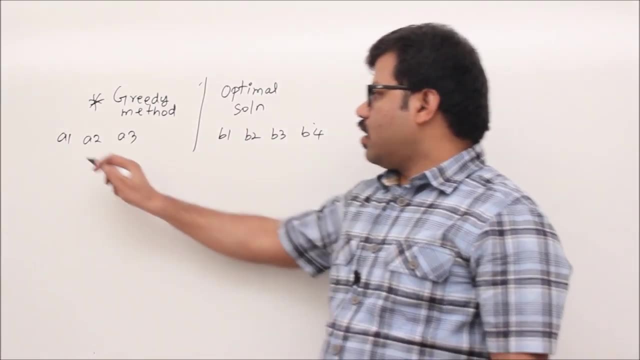 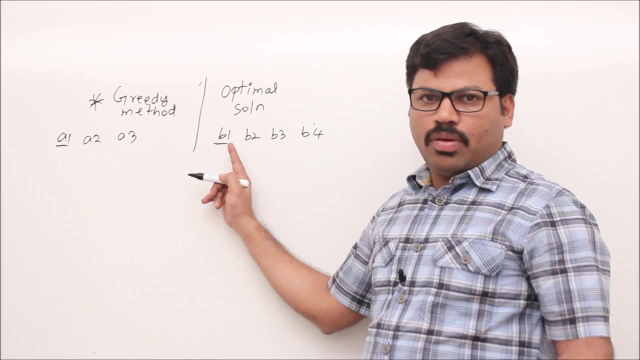 if they are same, then my greedy method also gives- I can say that- optimal solution. Now, at least one activity should be more than our greedy method. So I ask first question: A1 and B1, are they same? If A1 and B1 are same, then no problem. 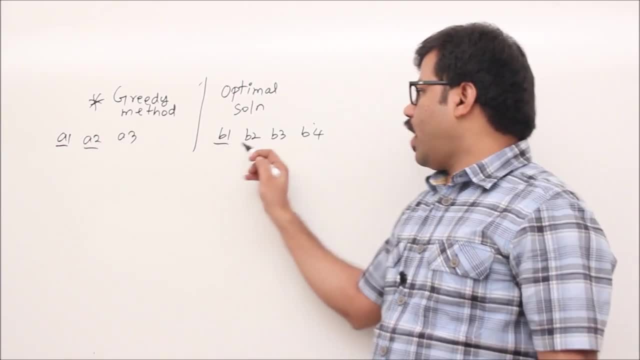 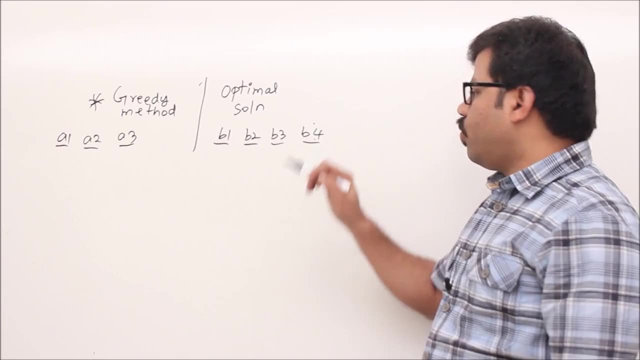 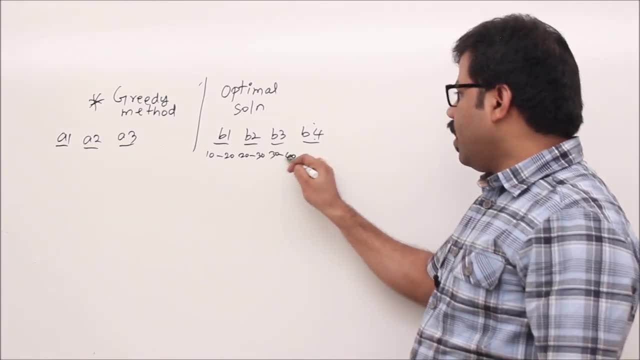 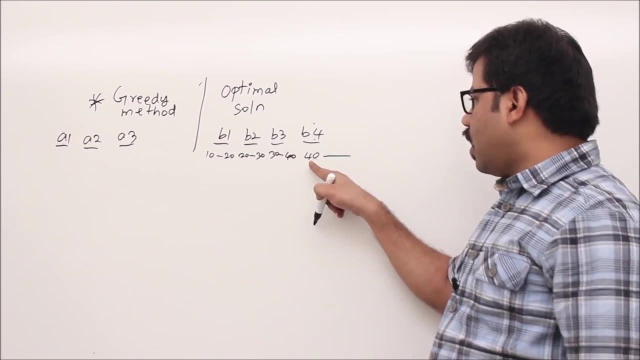 20, B2 20 to 30,, B3 30 to 40, then B4 is compatible with them, then it should be 40 to something. If you have an activity which starts after 40, then even that- I can pick here My greedy- 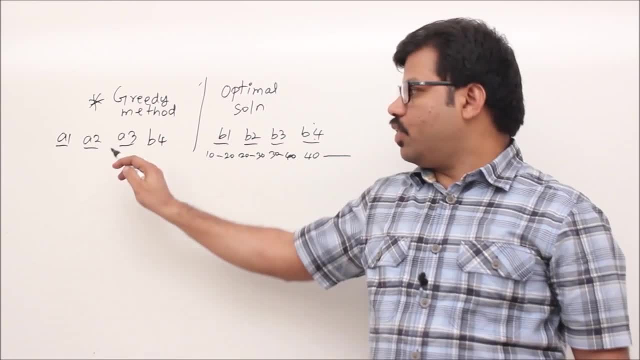 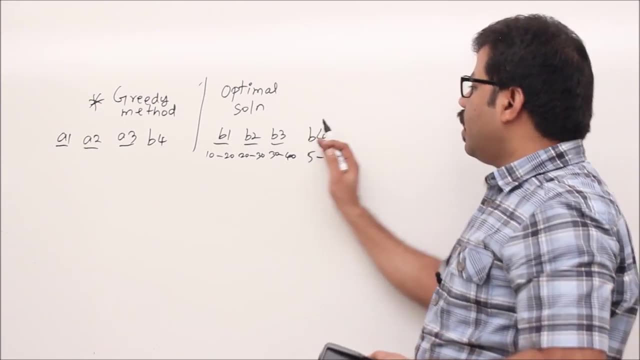 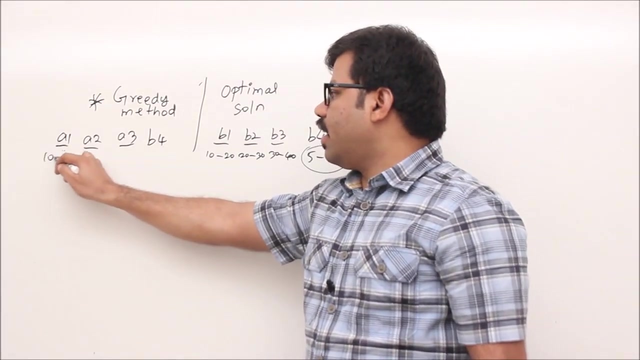 method also picks it Correct, Because we know the algorithm, just execute. you understand Now. so that is not the case, Then maybe B4 is from 5 to 10, it is left side of B1. Then if we have this kind of activity, then why I will pick A1, which is starting at 10?? 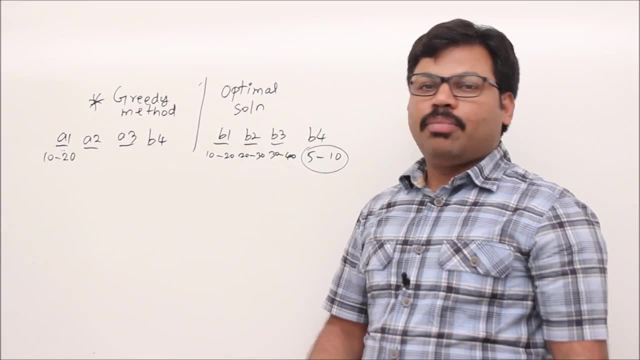 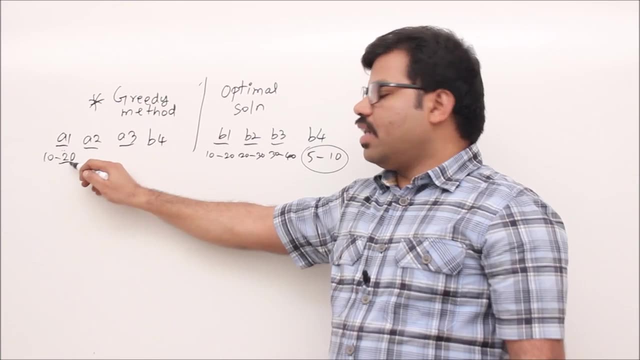 Because always I pick up. did you remember one thing? Strategy is picking up the activity whose finishing time is earliest. I thought A1's finishing time is earliest among all. That is why I picked it. Really, we have this kind of activity. 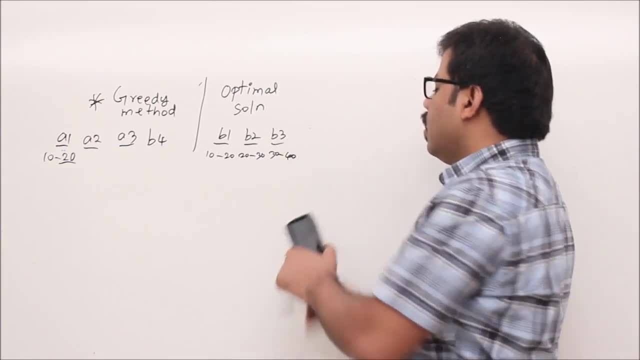 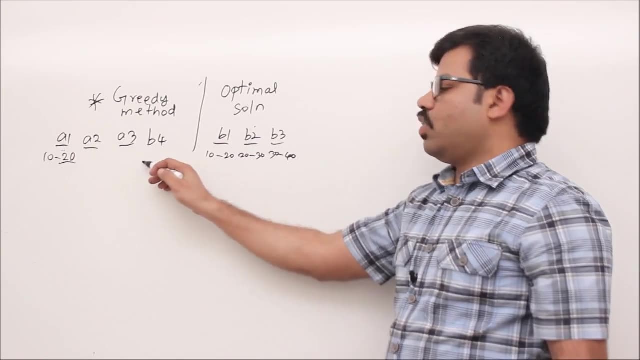 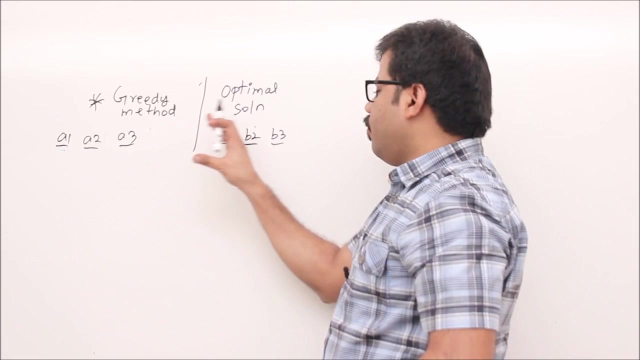 I would have taken it correct. So that is why it is impossible Then. so B4 kind of activity impossible. Then remove B4, then optimal solution and your solution are same. right Now you will see the second case where you are not matching A1, A2, A3 with B1, B2, B3. 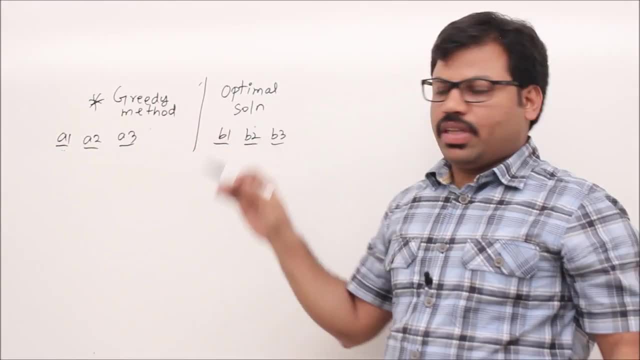 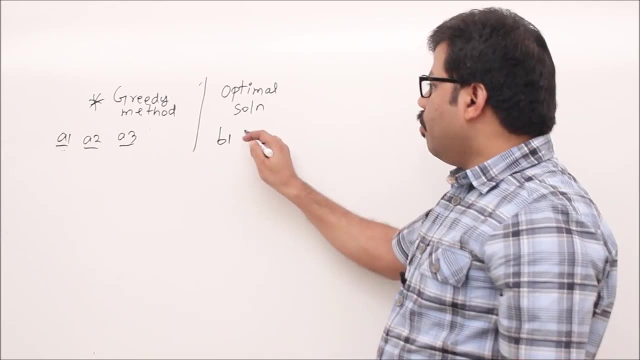 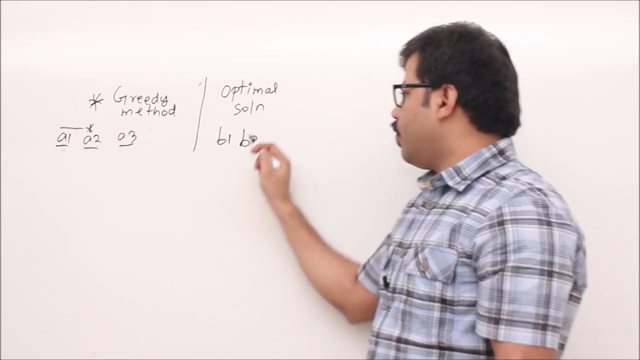 That means these activities are not matching with B1, B2, B3. Example A1 you have, he has B1, optimal solution has: both are same, But B2 is different from A2.. That means after some time in the activity list one activity is differing. 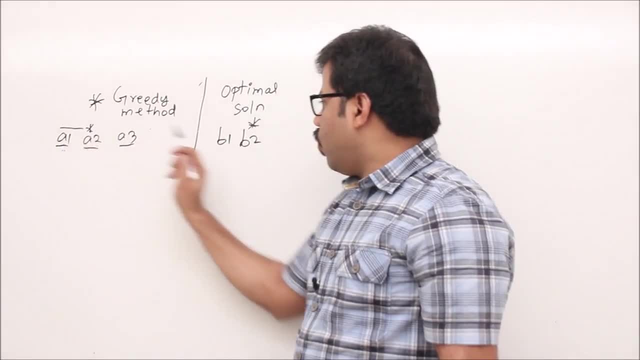 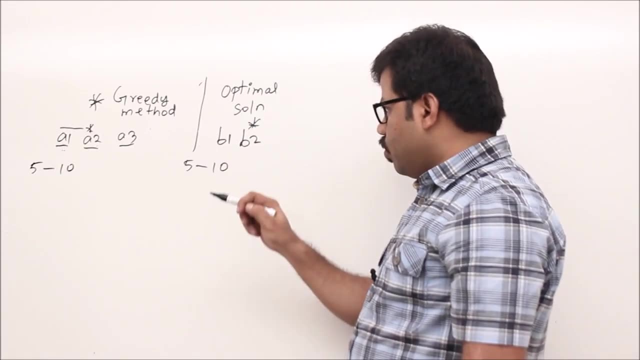 First time. Then I ask if A1 equal to B1, example: A1's duration is 5 to 10, B1's duration also 5 to 10.. Now I ask: B2, Mr B2, you are not. you are different from A2, then why? 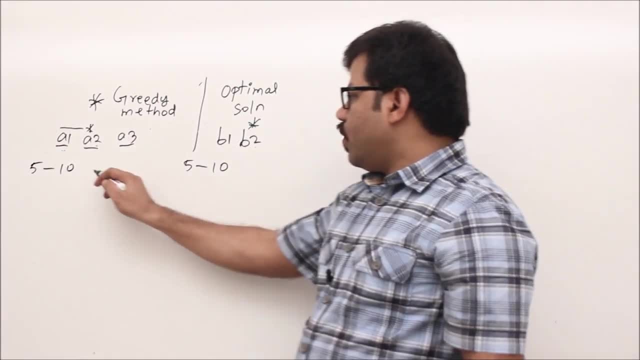 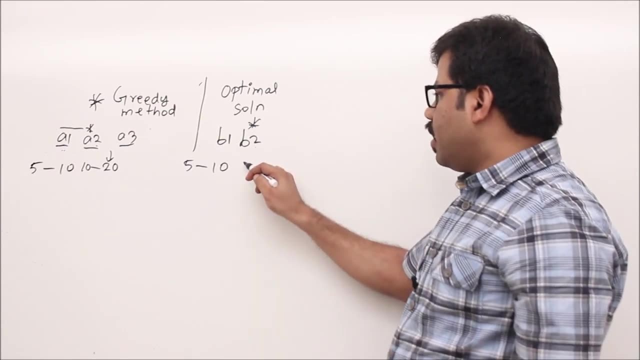 What is your finishing time? My A2's finishing time is, let us say, 10 to 20, that means 20.. Then B2's finishing time, let us say: either there are two cases, Maybe it is one case is something- 10 to 30..